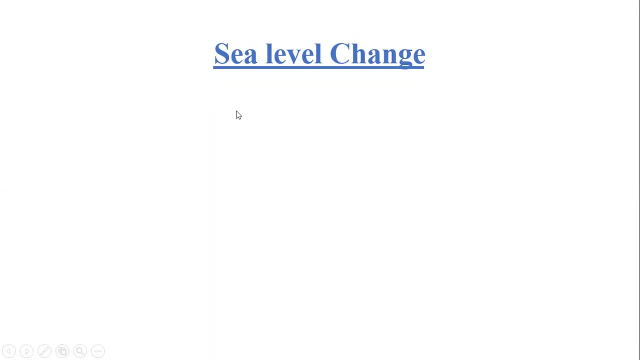 we are then unable to understand the stratal pattern as well as the sedimentary signature, or stratigraphic signature within the sedimentary rock record. As the sea level changes, it affects the sedimentation And the effects of sea level rise as well as sea level fall is induced in the form of stratigraphic signature in the sedimentary rock record. 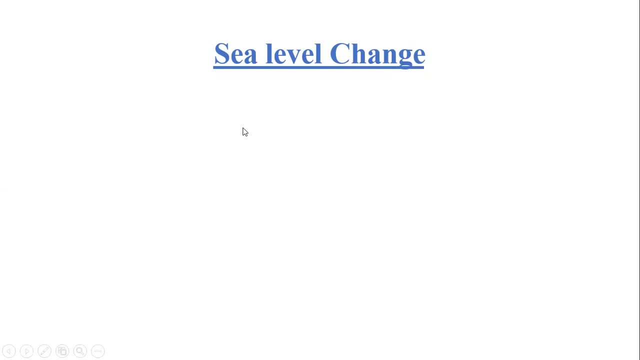 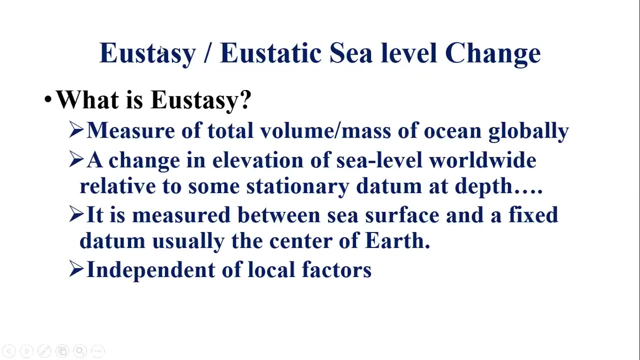 Therefore, understanding of sea level changes is essential for establishing sequence stratigraphy of any particular area. What is eustachy and what is eustachic sea level change? Eustachy refers to the measure of total volume or mass of ocean globally. 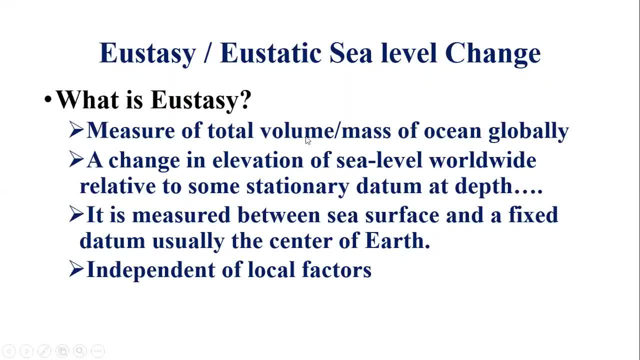 The measure of total volume or mass of ocean globally is termed as eustachy. Or a change in elevation of sea level worldwide relative to some stationary datum at depth is termed as eustachy. A change in elevation of sea level worldwide relative to some stationary datum at depth is termed as eustachy. 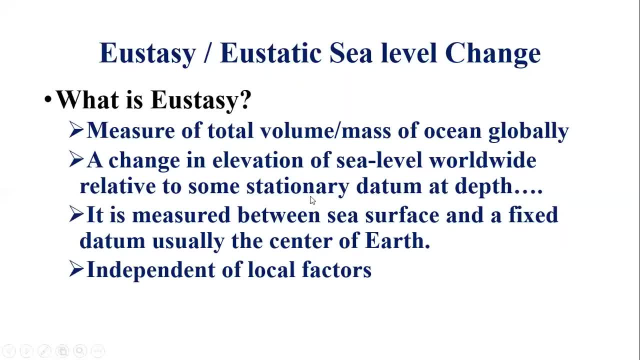 By stationary datum we mean a static datum or a static surface which is not prone to the movement, which is not affected by the tectonics and which doesn't move either upward or downward. It is measured between the sea surface and the thick datum. 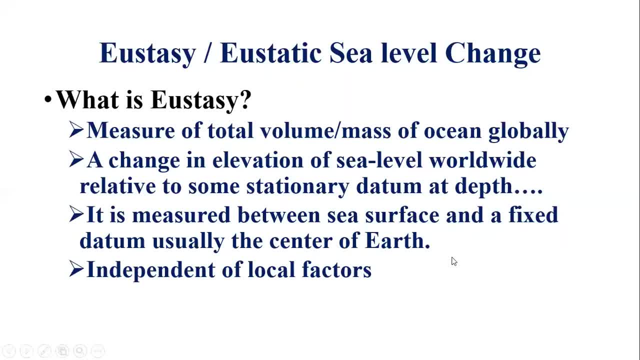 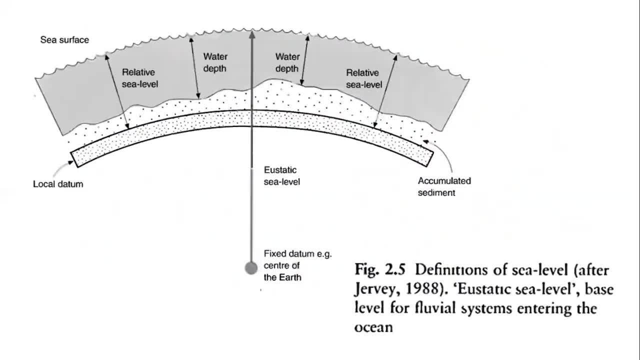 fixed datum is usually taken: the center of Earth. Eustachy is measured between the sea surface and the thick datum, usually the center of Earth. Here you can observe this is eustachy, or a static sea level. It is measured from the thick datum which is usually taken: the center of Earth. 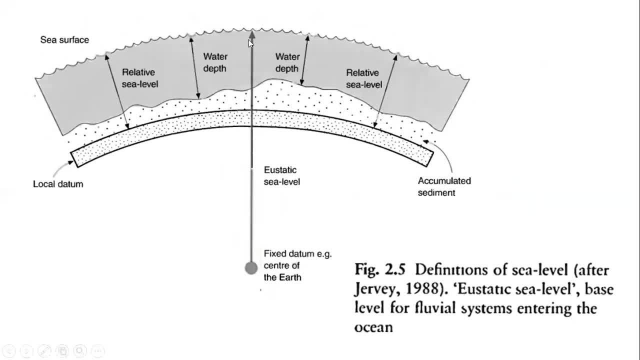 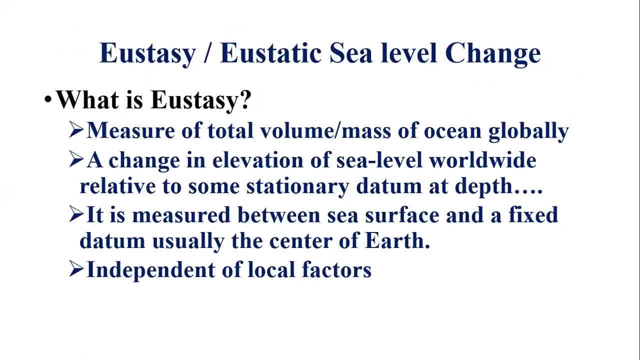 is taken as a thick datum from the center of Earth up to the sea surface. This elevation is termed as a static sea level. Static sea level is independent of local factors. Local changes occurring within the ocean doesn't affect the eustachy sea level. 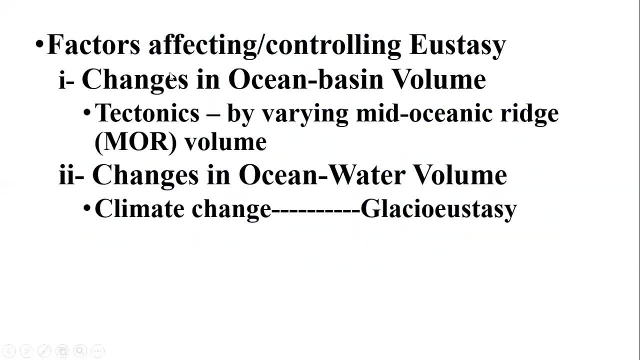 It depends upon or it is affected by the following five factors: First is changes in ocean basin volume. Second is changes in ocean water volume. Now how changes in ocean basin volume occur and how they affect the eustachy or how they control the eustachy. 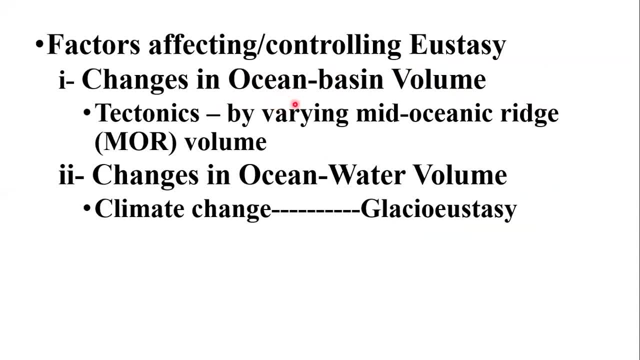 You know about the seafloor spreading which occur along the mid oceanic ridges, where new oceanic crust is created. So when mid oceanic ridges are active globally, then new oceanic crust is created as a result of seafloor spreading. 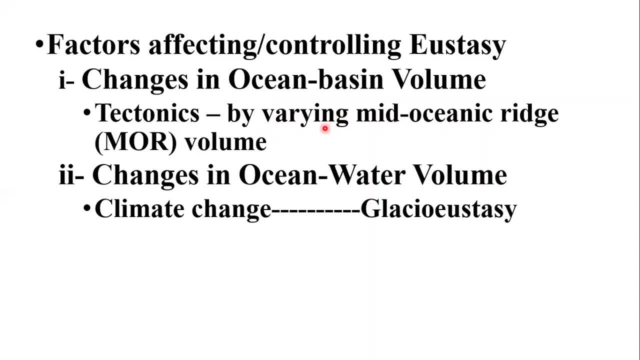 which results in the increase in ocean basin volume, And when ocean basin volume changes as a result, water present within the ocean basin also gets affected. Ocean basin, the water volume present within the ocean basin, is also affected by the changes in ocean basin volume. 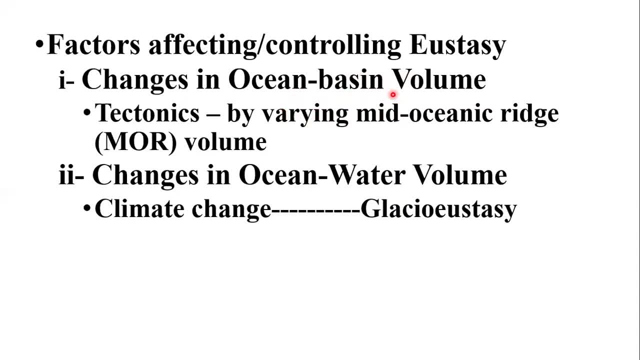 And in this way ocean basin volume changes. the eustachy Now how changes in ocean water volume occur. It occurs by the climate change, And climate change is induced by the global warming. Global warming results in two phenomena. First is due to increased temperature of the worldwide. 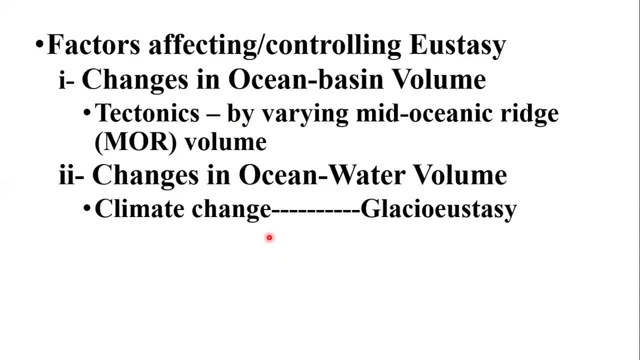 expansion of oceanic water occur. Water of ocean expands due to the increased temperature, While second phenomena- and remember that as expansion of water volume of ocean water results in the increasing the sea level- And due to increased temperature, ocean water expands and thus rises the sea level. 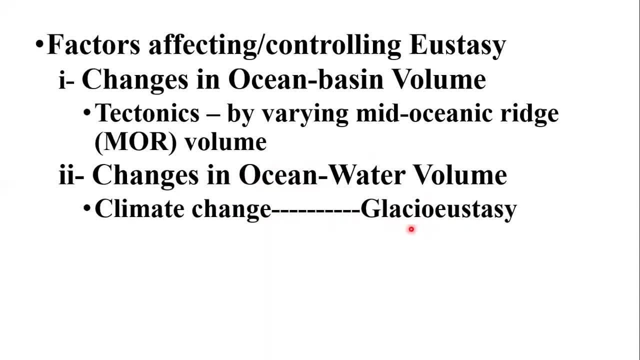 Now, what is glacial eustachy? This is second phenomena which occurs due to the global warming. You know about the glaciers, that glaciers are present on the continent in the form of ice sheets. are the continental glaciers When global warming occurs? 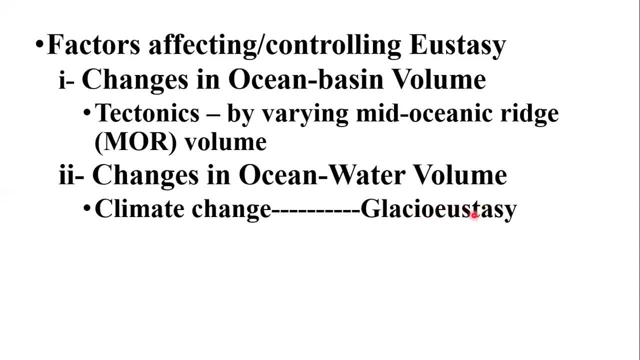 these glaciers melt. As a result of melting of glaciers, you know that the final place of melt water is ocean. They fall into the ocean. So when, if the whole or major portion of continental glaciers get melted, then more water is released or more water falls into the ocean. 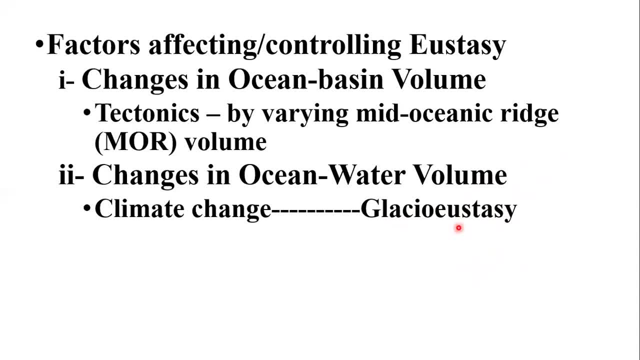 As a result, the ocean water volume increases, Thus increasing or raising the eustachy, Or it increases the global sea level. So in this way, climate change affects the ocean water volume. First is expansion of water due to increased temperature worldwide. 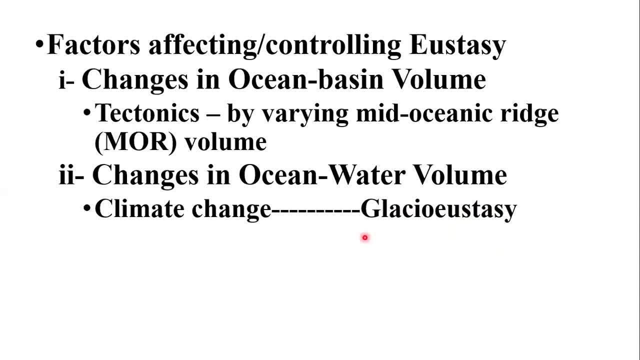 Second is the melting of glaciers. On other hand, if global cooling occurs and there is ice age, may majority of the water present on the earth is in the form of glaciers due to ice age, then global sea level fall occurs, And we say that this is eustachic fall. 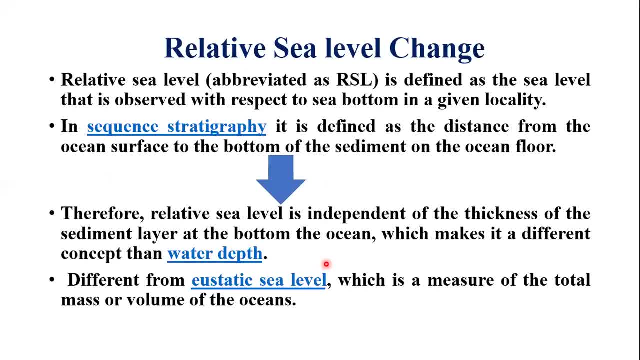 or fall within the eustachy. What is relative sea level change? Relative sea level change is defined as the sea level that is observed with respect to the sea bottom in a given locality. Eustachy is the global sea level change, while relative sea level is observed. 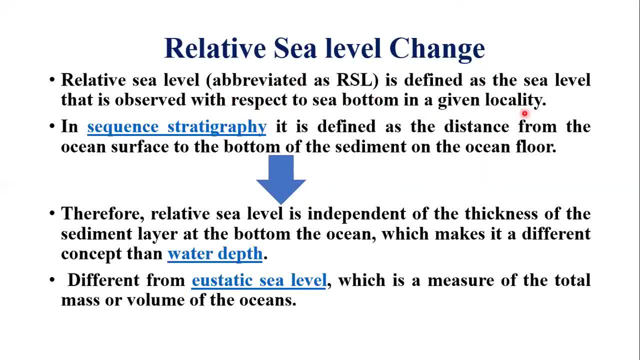 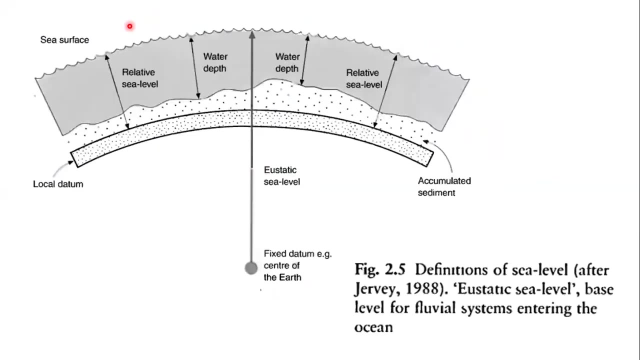 with respect to the sea bottom in a given locality. It is measured or it is observed locally In sequence stratigraphy. it is defined as the distance from the ocean surface to the bottom of sediment on ocean floor. You can observe here in this diagram: 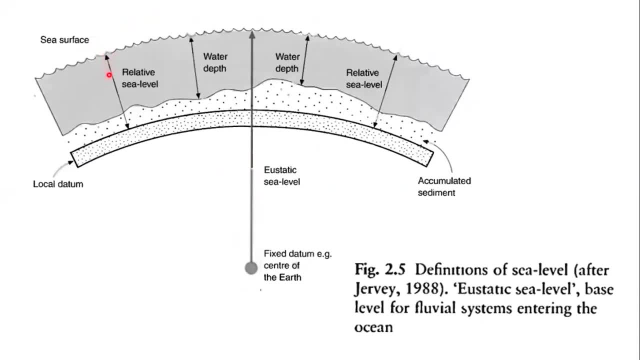 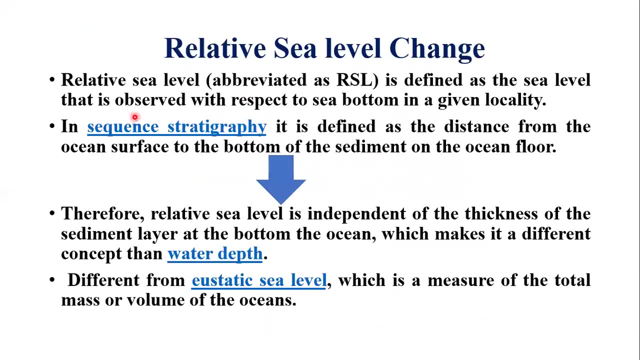 the distance measured between the sea surface and the bottom of sediment. This elevation or this height of water is termed as relative sea level. The relative sea level is independent of the thickness of sediment layer at the bottom of the ocean, which makes it different concept. 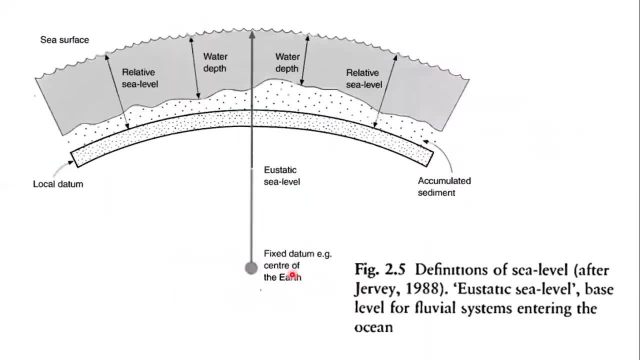 than the water depth. Now, what is difference between the water depth and the relative sea level? Relative sea level is measured from the sea surface to the bottom of sediment pile present on the ocean floor, While water depth is measured from the sea surface to the top of the sediment pile. 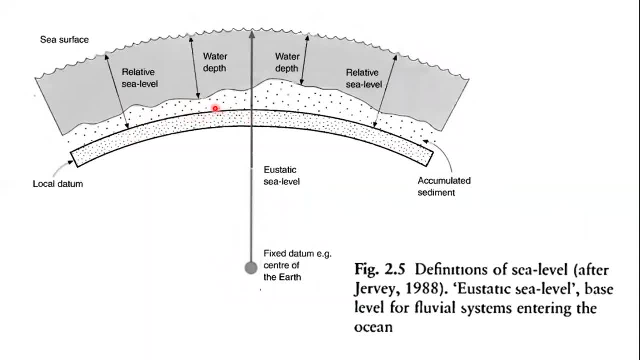 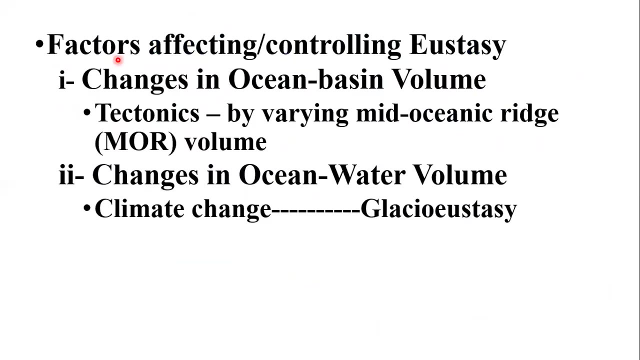 present on the ocean floor. So this is the difference between the relative sea level and water depth. One is measured from the top to the surface, while another is measured from the bottom of sediment pile to the surface. It is different from to static sea level. 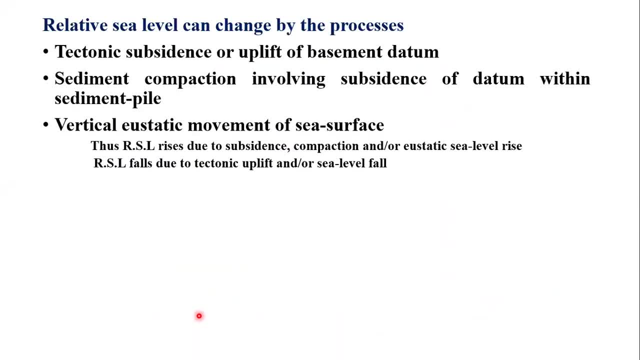 which is measure of the total mass or volume of the ocean. Relative sea level changes by the following process: First is tectonic subsidence, or uplift of basement datum. Second is sediment compaction, involving subsidence of datum within the sediment pile. Third is vertical eustatic movement. 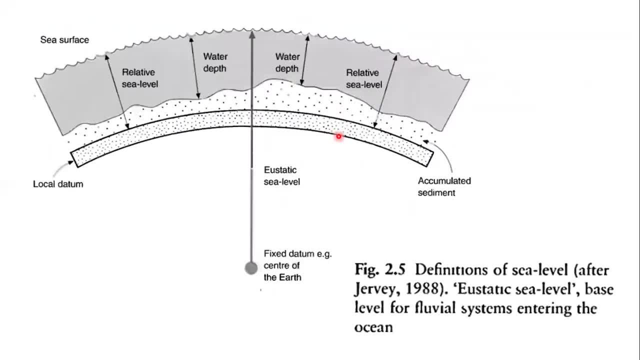 of sea surface. If this datum either subsides or either are uplift due to the tectonic, then the relative sea level changes. If it subsides, if it moves downward due to tectonic activity, then the relative sea level rise will occur. Another end: if it gets uplifted. 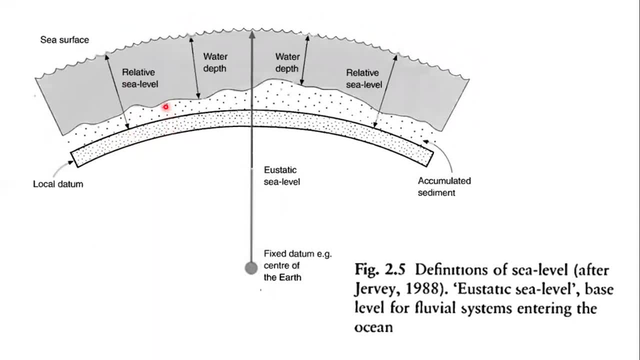 the uplift of this datum occur, then you can observe that, as a result of uplift, the relative sea level fall will occur. the elevation will decrease from the surface to the bottom if this surface gets uplifted gets uplifted. Second, is the sediment compaction involving subsidence of datum. 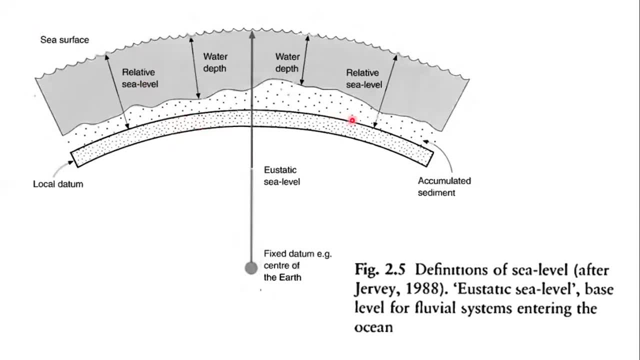 within the sediment pile, If any. if a datum is considered within the sediment pile, if this surface is considered and as a result of sediment compaction this layer also subsides, then as a result of sediment compaction, sea level or relative sea level rise will occur. 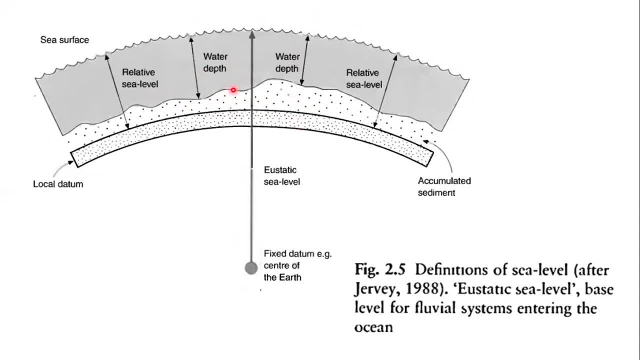 If there is vertical eustatic sea level. if there is vertical eustatic movement means that vertically sea level changes. by vertical sea level changes we mean that eustatic sea level rise occur. rise within the eustacy occur then due to eustatic sea level rise. 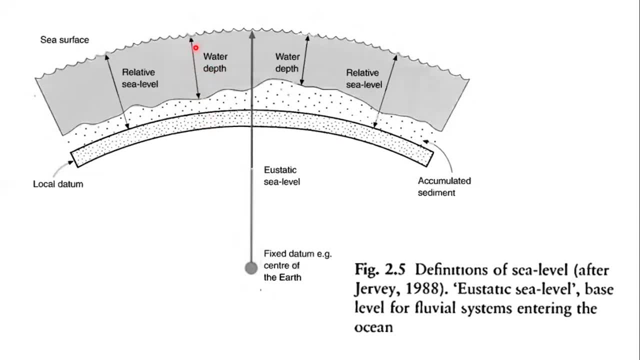 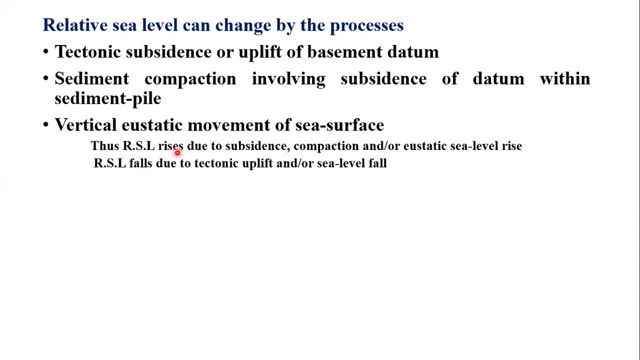 relative sea level rise. relative sea level also rise, so we may say that sea level- relative sea level- rises due to subsidence, compaction and or eustatic sea level rise. subsidence plus compaction or and eustatic sea level rise results within the relative sea level rise. 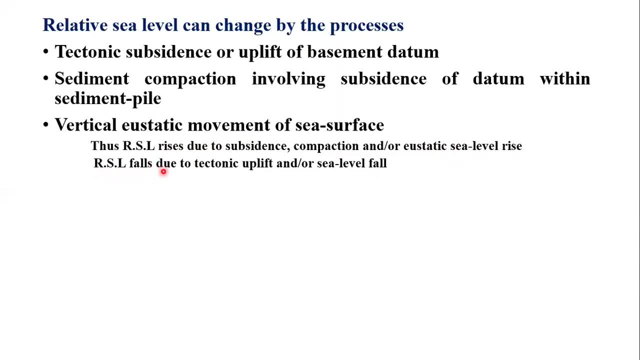 another end. relative sea level falls due to tectonic uplift and or sea level fall. if there is eustatic sea level fall, then when globally- eustatic, globally sea level is falling, then locally sea level will also fall and as a result of eustatic sea level fall. 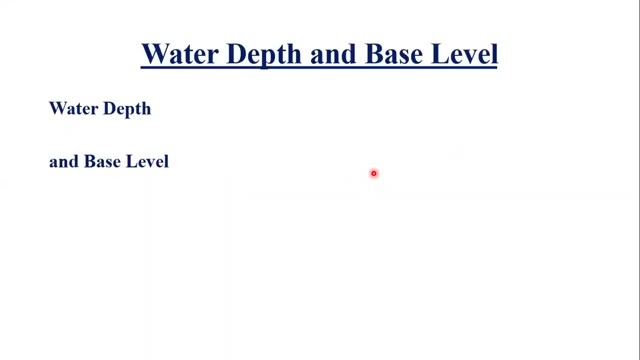 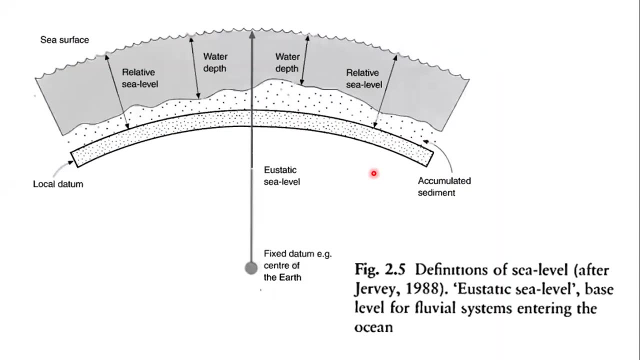 relative sea level fall will occur. now, what is water depth and base level? we discuss the water depth. water depth is measured between the sea surface and sea bed in any given locality or any given point. it is measured between the sea surface and the sea bed, or, or in other words, 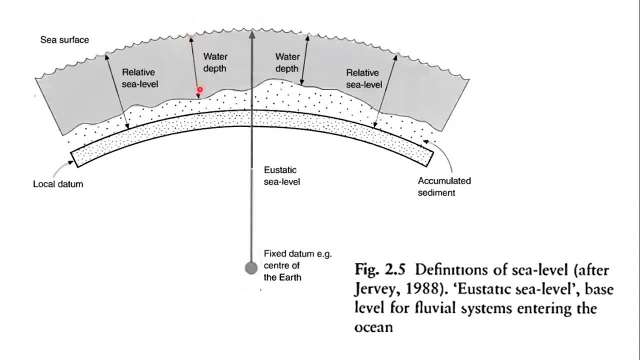 water depth is the elevation from the sea surface up to the top of sediment pile, and this is difference between the relative sea level and water depth. water depth is measured up to the top of sediment pile, while relative sea level is measured from the sea surface up to the base of the sediment pile. 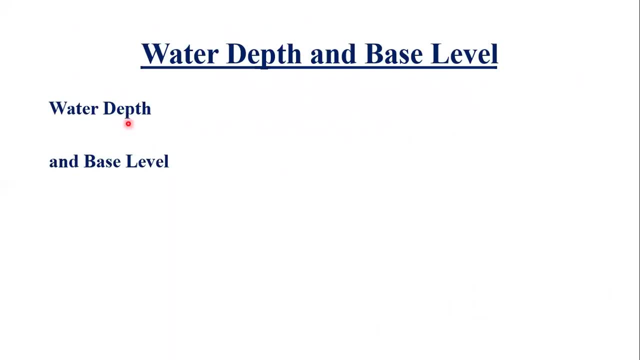 what is accommodation? what is base level? base level refers to that level, that surface above which deposition is temporary and erosion occurs. it means that base level is a level below which deposition can occur, but above which, if deposition occurs, then that deposition is temporary and it is usually eroded. 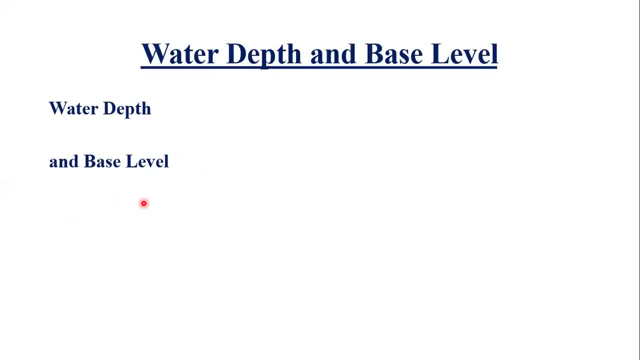 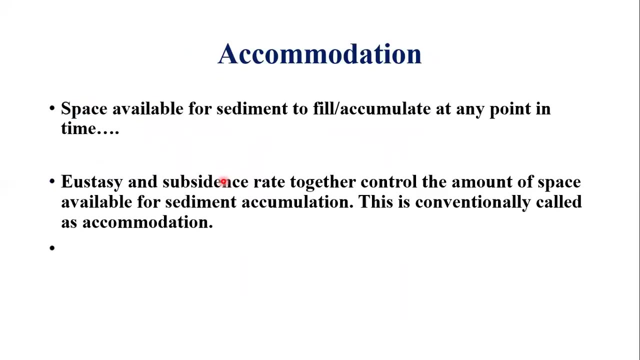 so the level above deposition, above which deposition is temporary, is termed as base level. what is accommodation? accommodation refers to the space available for sediment to fill or accumulate at any point in time is termed as accommodation. now, what controls the accommodation? first of all, the base level. base level. 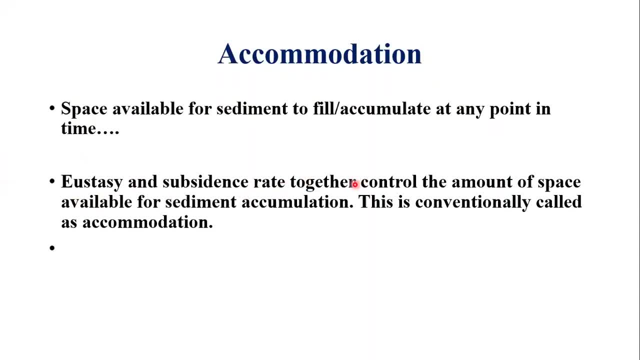 controls the accommodation. first is eustachy and subsidence rate. they together control the amount of space available for sediment accumulation, and this amount of space available for sediment accumulation, which is controlled by the eustachy and subsidence rate, is conventionally called as accommodation. 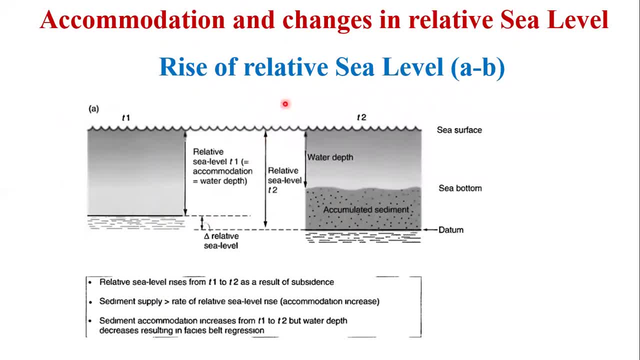 in these diagrams we will try to discuss that: how accommodation is affected by the changes in relative sea level, how the base level is affected by the relative sea changes in relative sea level and how water depth is affected and what is the effect of rate of sediment supply. 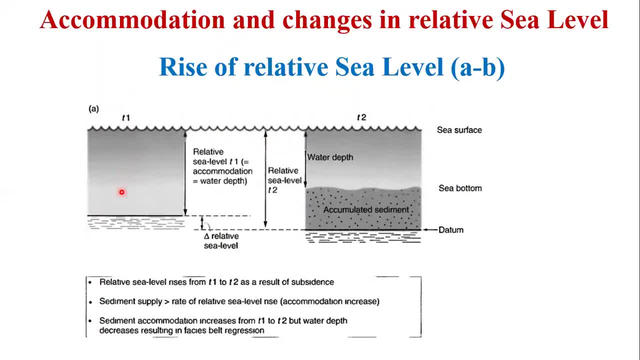 here you can observe, this is the sea level in time t1 and here you can observe that the relative sea level, as well as the accommodation, accommodation heat. described the accommodation earlier, that it is the space available for sediment accumulation in time t1, the relative sea level. 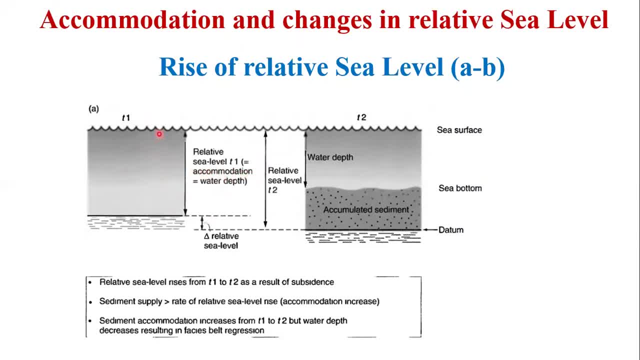 is equal to the accommodation, as well as equal to the water depth, so these three are equal. in this time- t1- now in time t2- subsidence occurs. subsidence of this datum occurs now when the subsidence occur. we know that subsidence results in the rise of. 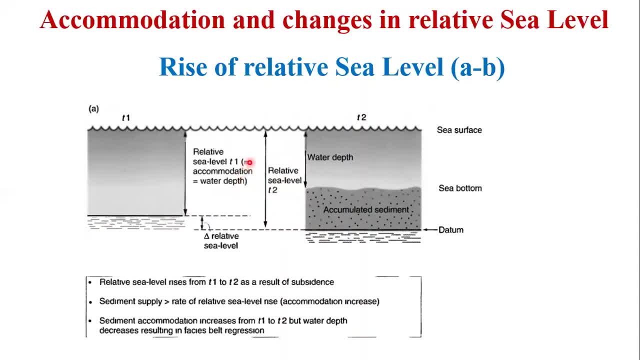 relative sea level. so relative sea level has rise than from t1 to the t2. but here you can observe that the sediment supply is greater as compared to the rate of relative sea level. so when sediment supply is greater than the relative, then the rate of relative sea level 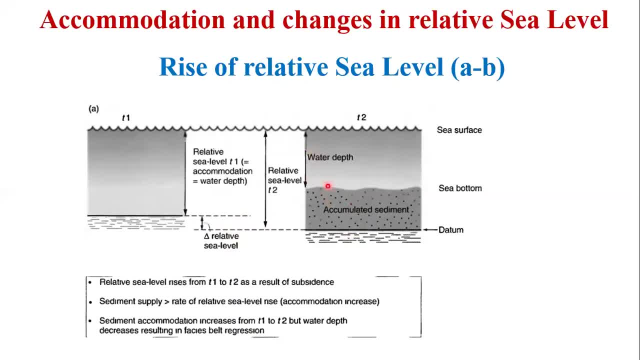 then water depth decreases. you can observe here that water depth refers to the distance from the sea surface to the top of sediment. so here, due to subsidence, accommodation has increased. relative sea level has increased, but due to high rate of sediment supply, water depth has decreased. another end: 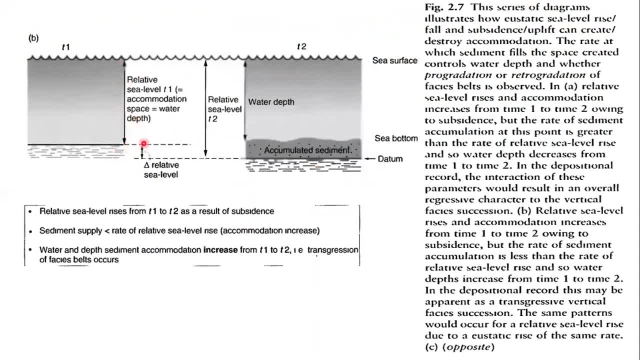 here you can observe that, due to subsidence, relative sea level has increased, but the rate of sediment supply is less than the rate of relative sea level rise. so here water depth has increased due to the relative sea level, because the rate of sediment supply is less than the rate. 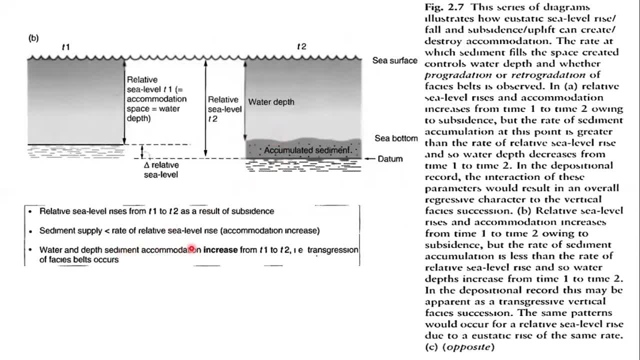 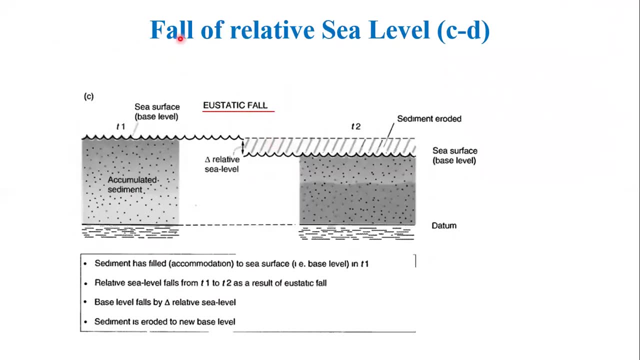 of relative sea level rise. so here transgression of fishy belts will occur. here in this diagram we will discuss that how fall of relative sea level affects the accommodation space and how it affects the water depth and how base level is affected. here you can observe that relative sea. 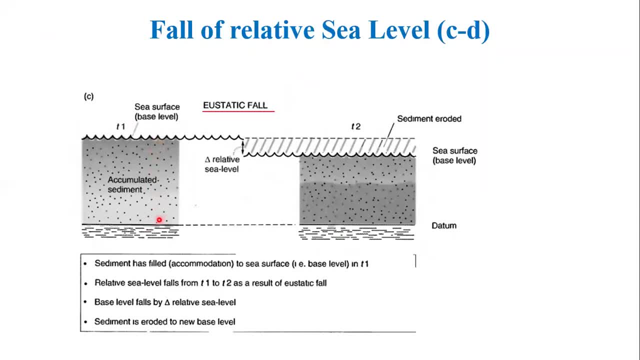 level is at this position in the time t1. this is sea surface. now, if sea level fall occurs due to some geological reasons, and these are the accumulated sediment, and you can observe here that sediment has filled the accommodation space. there is no space left for other other sediments to accumulate. 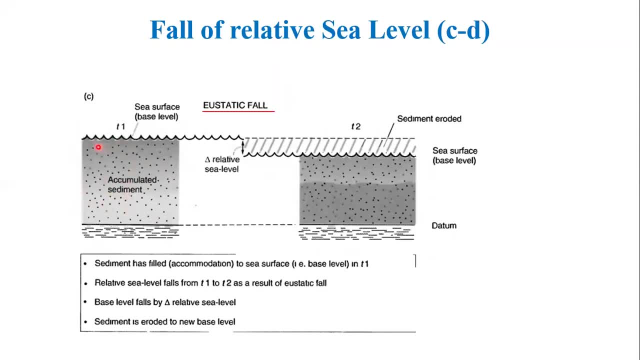 so here you can observe that this is base level. above this level, sediment deposition will temporary and it will erode away. so when relative sea level fall occurs, this is the rate of relative sea or change of relative sea level fall. relative change now as a result of: